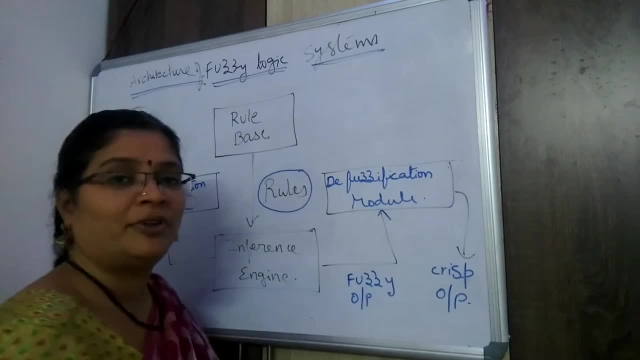 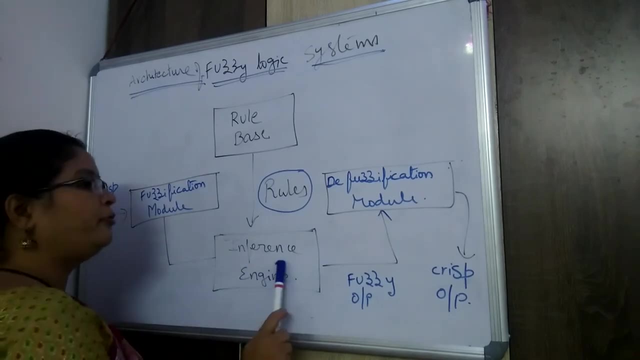 Let us see in this diagram. these are the components of the purgy logic system architecture. The first one is nothing but rule base purgification module, inference engine, defurjification module- Here the crisp input will be given. And then here the crisp input will be given. 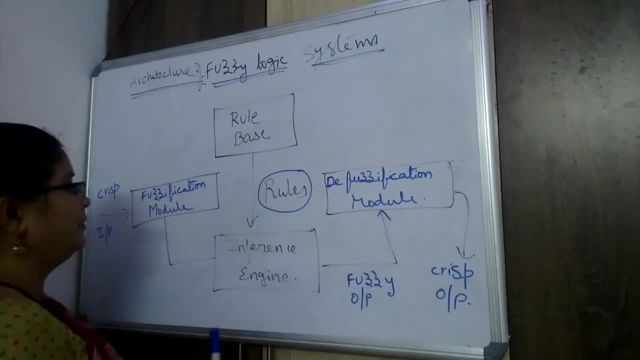 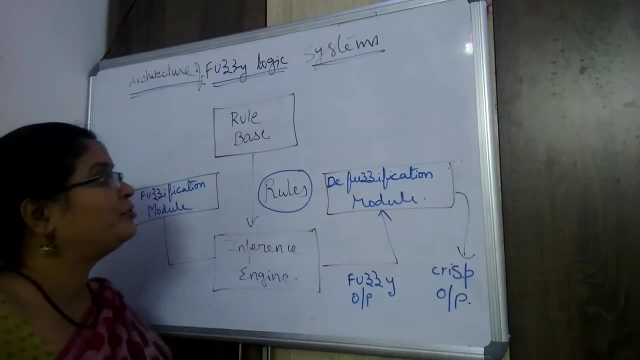 And then here the crisp input will be given, And then here the crisp output will be given, Here the purgy output will be there. Okay, so like that, the entire architecture will be represented. First of all we are going to see. the first one is nothing but the rule base. 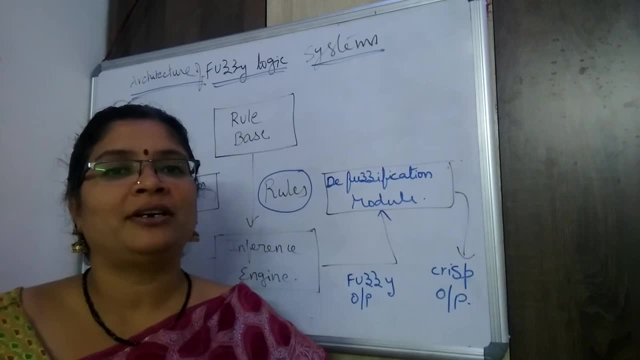 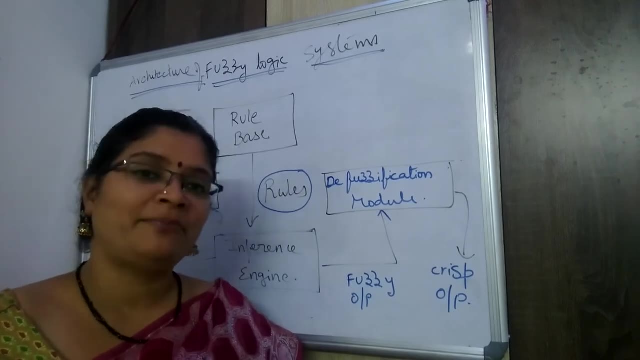 What is the meaning of the rule base? A rule is nothing but the thing to be followed, based on certain conditions, as in the real world. meaning of the rule? In the same manner, the rule in the purgy logic system also, whatever system developed by the experts. 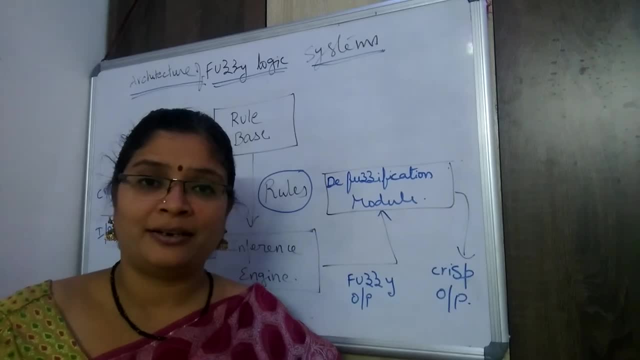 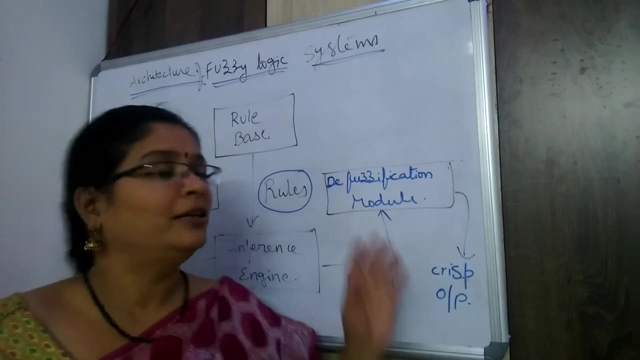 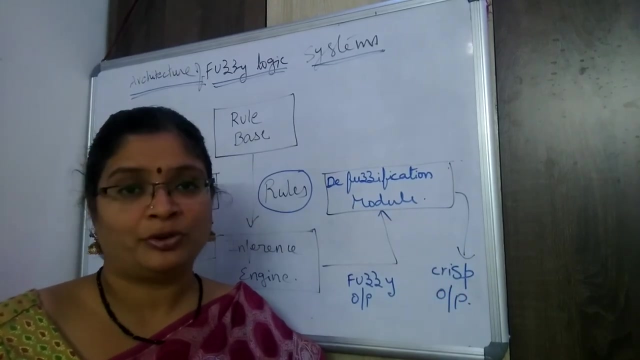 they will design some set of the rules. that means these certain numbers of the values will be allowed. Only the range of values from here to there will be allowed. Like that, they will put some rules, They will put some conditions on that. based on that, they will design certain number of the rules. 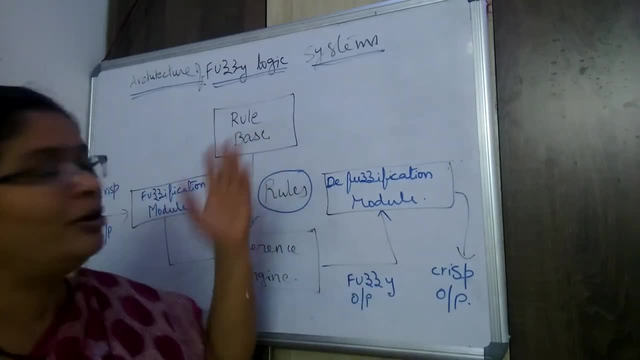 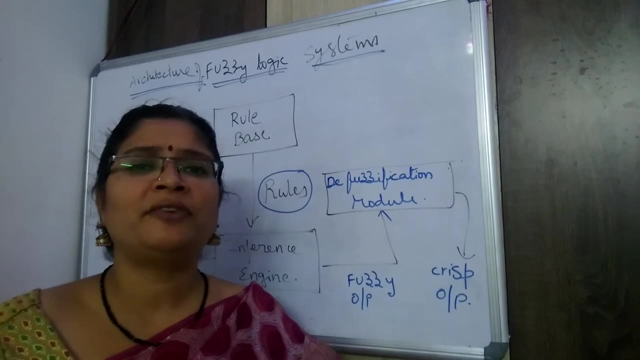 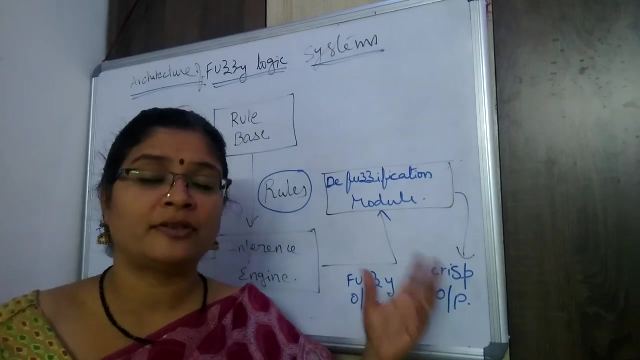 And where we store all these rules is nothing but the rule base. For example, the height of the person will be allowed from 3 to 6 feet and as well as the age of the person will be allowed, allowed from some 18 years to the 60 and above. okay, so 70 up to 70. okay, so we can measure the. 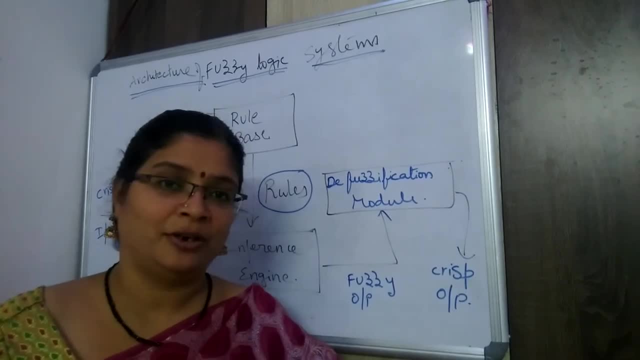 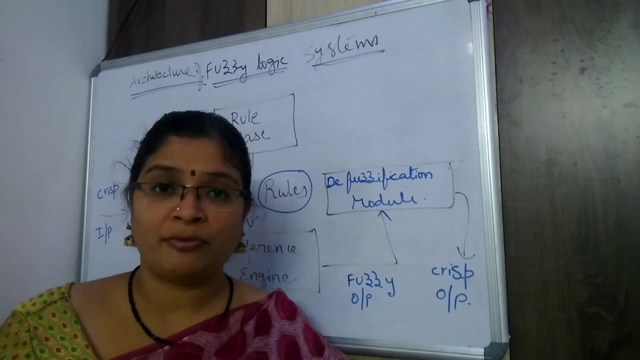 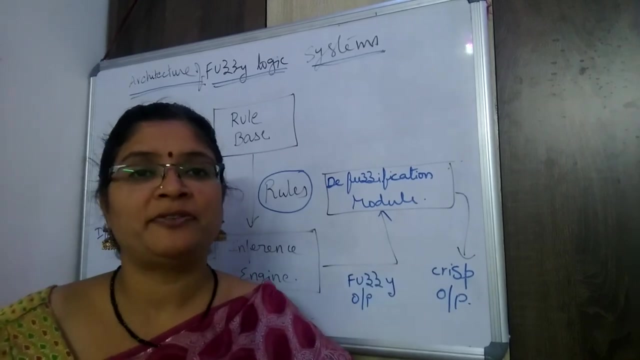 age of the person also some 38 years, 12 months like that, okay. and the salary of the person is allowed 4.5, 45.5 k, 45.6 k, like that, the continuous values that can be measured within a given range. the range will be specified by designing the rules and some conditions also we will apply on that. 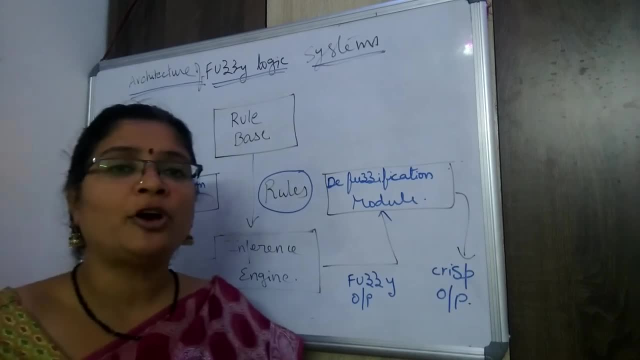 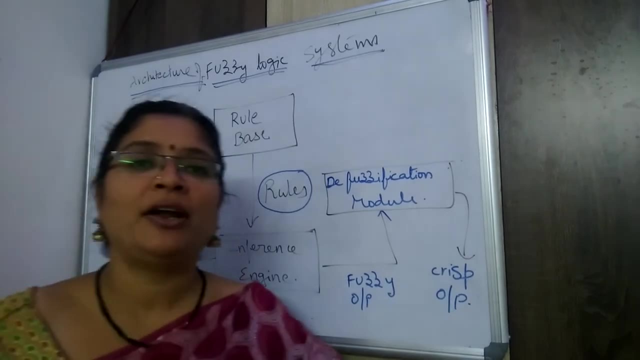 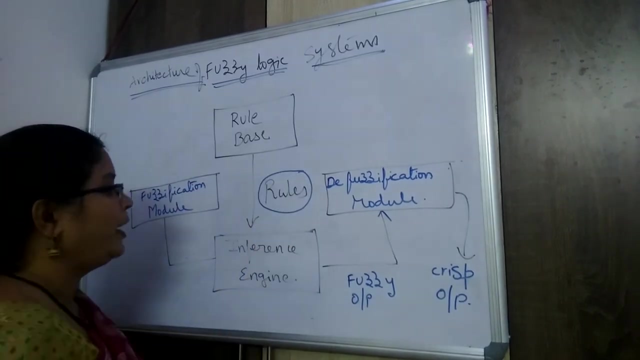 in the fudgy architecture, fudgy logic systems we put all such kind of the rules, whatever we have designed, in the root base. the root base is one of the important one which stores all these kind of the rules next. so that's why i have given here as the rules: okay, and these rules can be stored in. 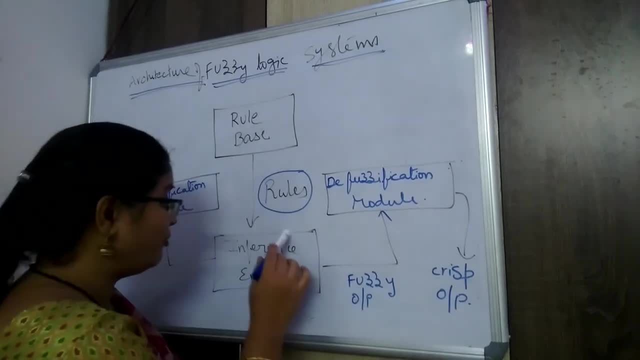 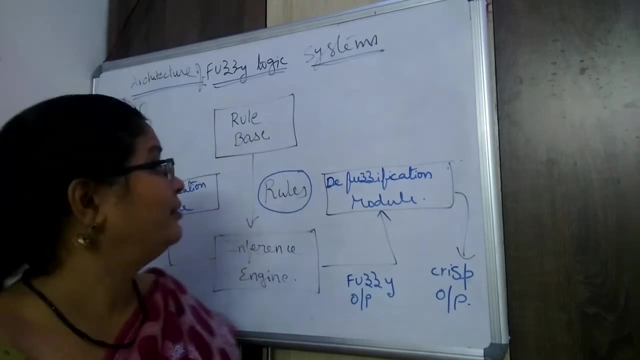 the inference engine. inference engine is a one of the important rules in the inference engine so that's why i have given here as the rules okay component which going to process all those rules. whatever the rules we put in our root base, that will be processed in the inference engine. that will be processed for a respective input to the 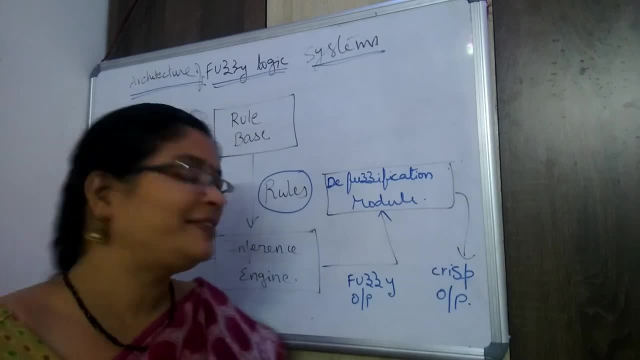 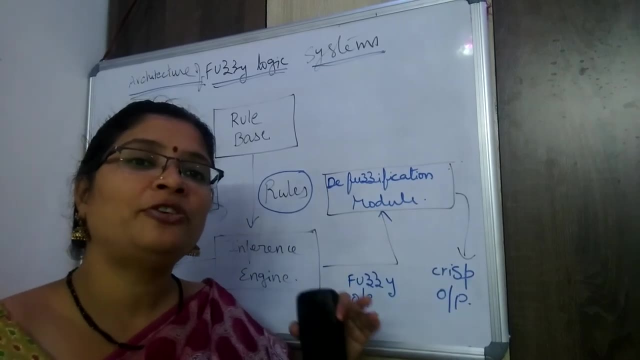 respective output, how it will be given. based on the rules, this is the activity of the inference engine. okay, so, if at all, certain input will come. so, based on the application of the rule, what kind of the output will be transformed to this modules? that will be decided with the help of the 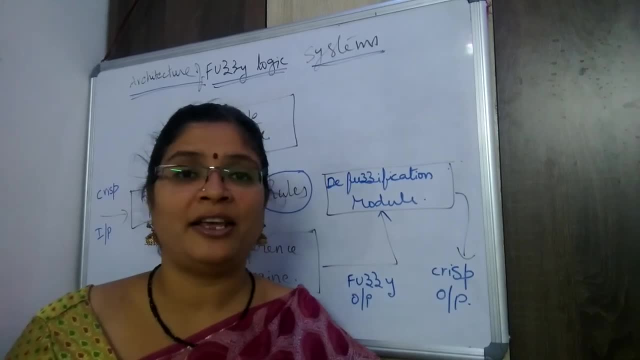 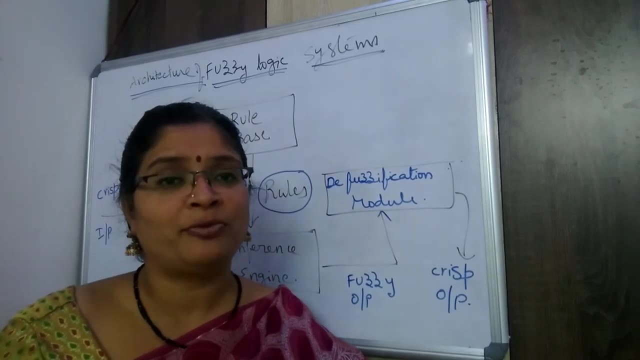 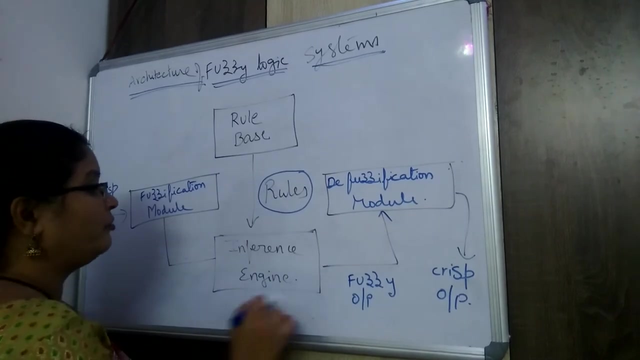 inference engine. inference engine is designed in a way to process all the rules based on the inputs and to generate what kind of the inputs and to generate what kind of the outputs. for getting what kind of the inputs, for generating what kind of the outputs. that is the activity of this particular. 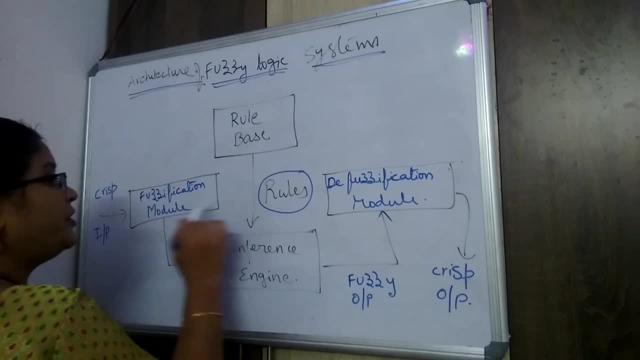 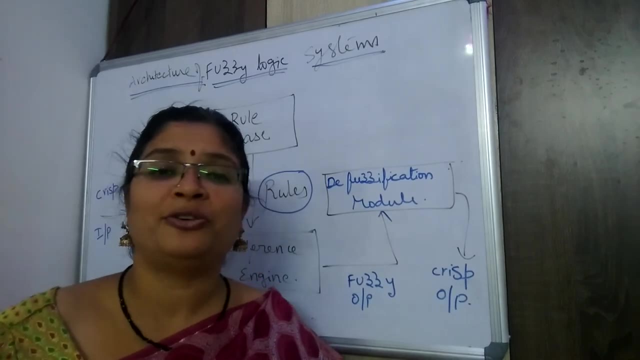 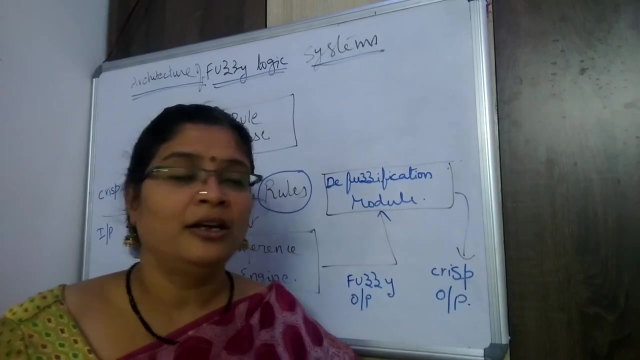 inference engine. okay, and now coming to the fudgification and defergification modules. before going to discuss about the fudgification and defergification modules, let us once again know what is the meaning of the fudgification. let me explain what is the meaning. 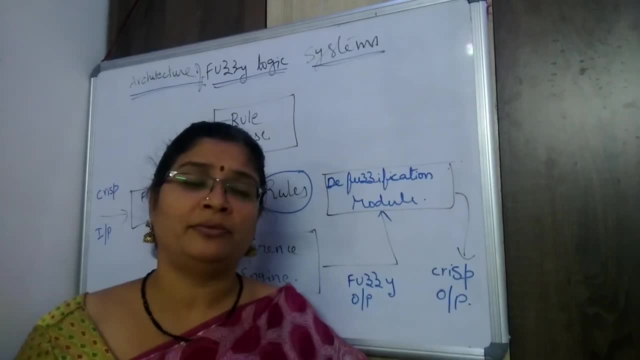 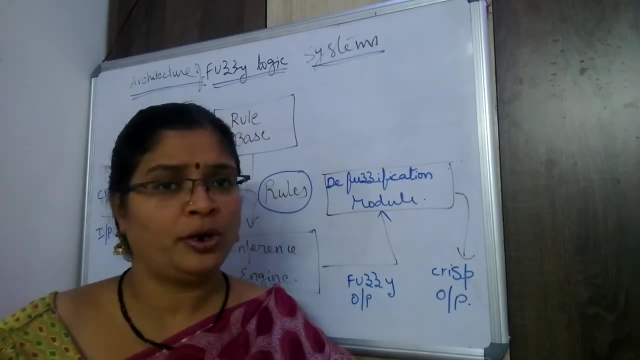 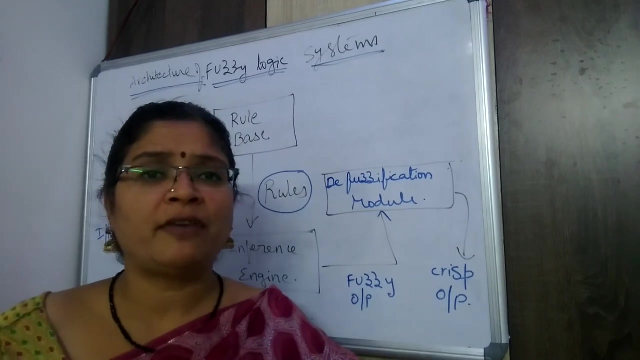 of the fudgification, whatever input that we will give. what kind of the input that is there? that is Boolean input. that Boolean input is also called as the CRSP input. okay, so the Boolean input that will be converted into the fudgie in output. okay, so CRISPR data will be. 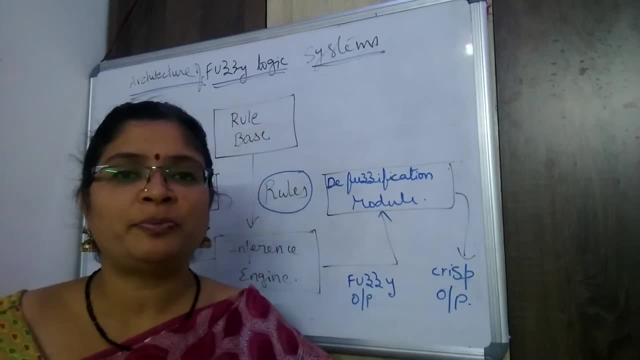 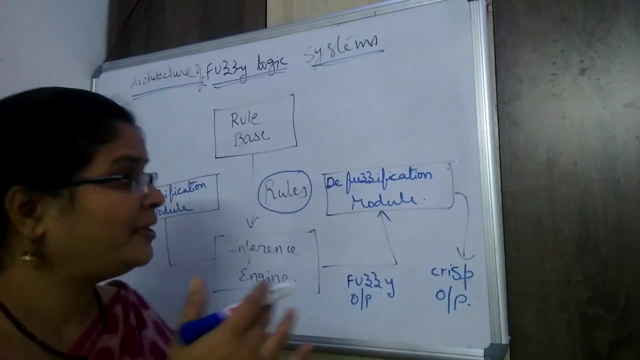 converted into the fudgie data. that means the CRISPR data can be categorized into the rays of light of the fudgy. This feature is called the fudgification. Okay, So what is the meaning of the de-fudgification? 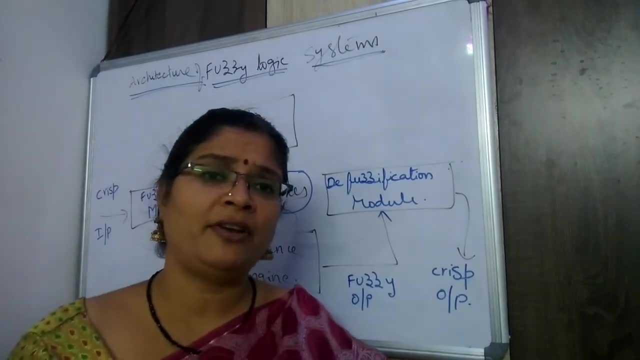 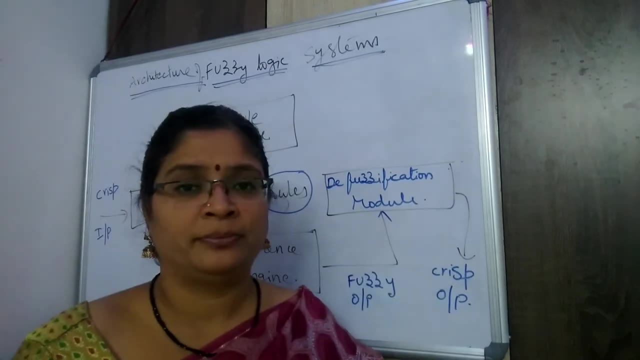 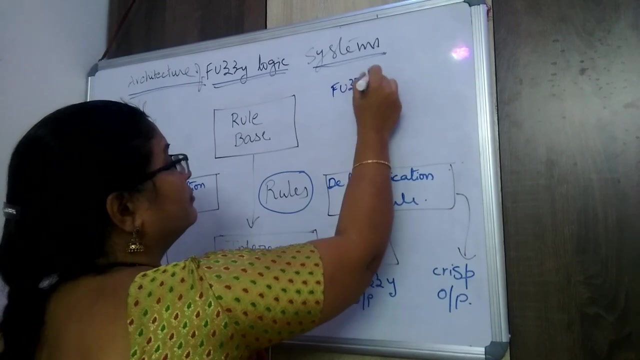 Whatever fudgy data will be there, whatever vague data will be there, that will be transformed in the crisp data- either true or false, either 0 or 1, like that. That is the meaning of the de-fudgification, So crisp to fudgy is called as the fudgification Fudgification. 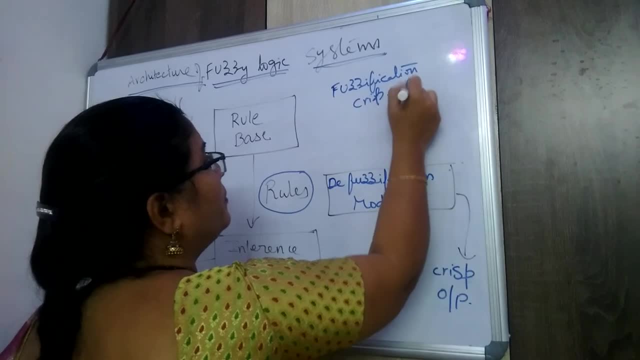 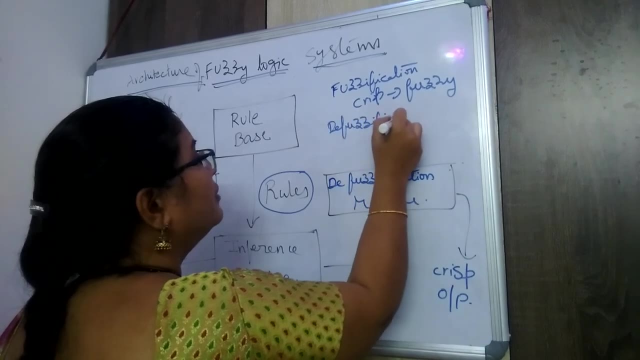 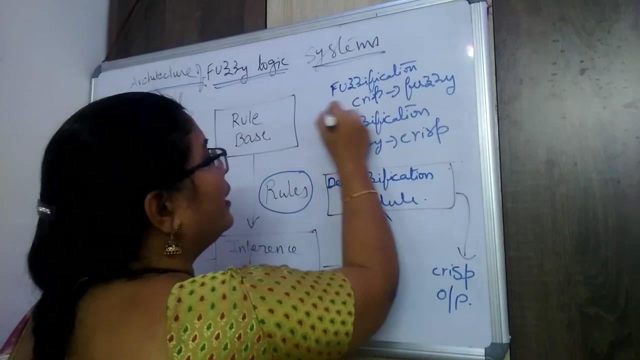 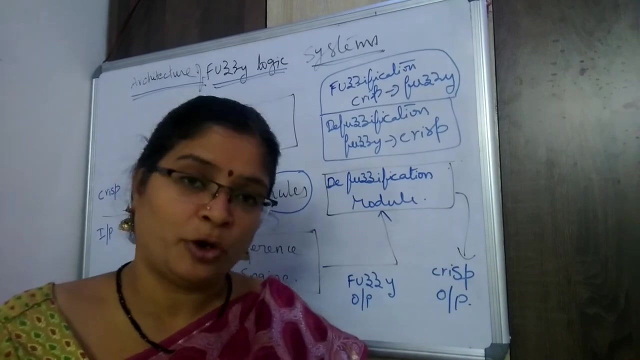 is termed as crisp to fudgy and de-fudgification is termed as fudgy to crisp. Like that we are having specific definitions of the fudgification and as well as the de-fudgification. Okay, So whenever we are getting here the input as the crisp input, Okay. 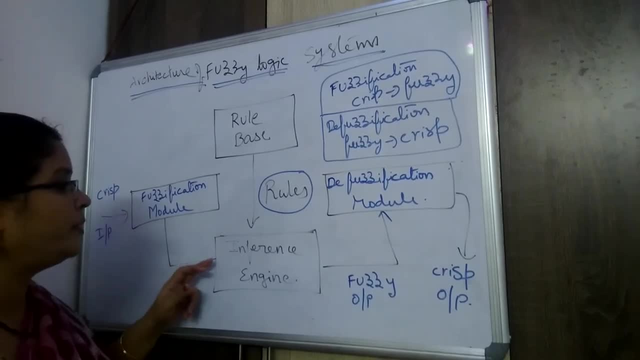 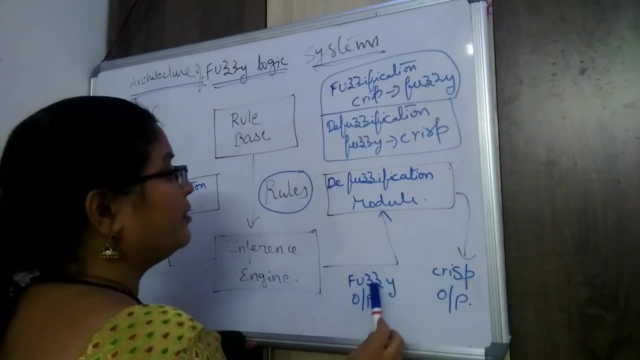 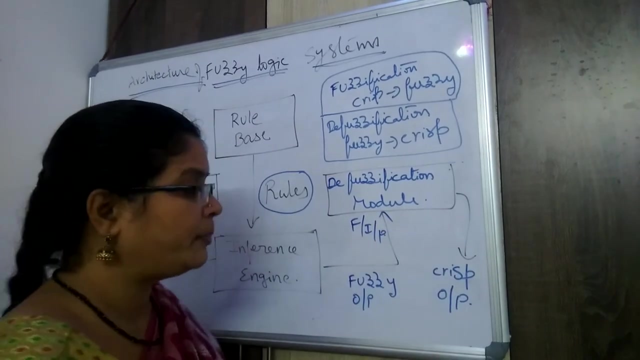 So this crisp input is fudgification and this will be go to the fudgy output. Okay, And here we are getting the de-fudgification module. It takes the fudgy input here- See here, it takes the fudgy input here- and this fudgy input will be transformed into the respective 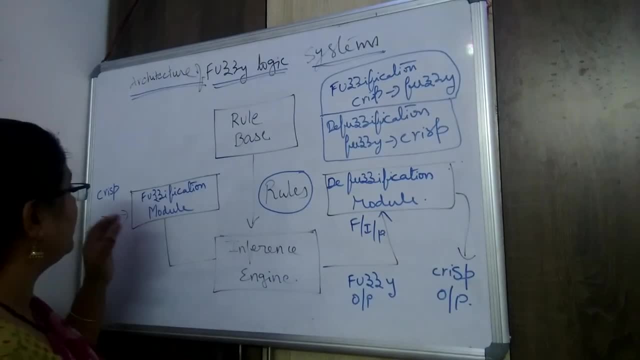 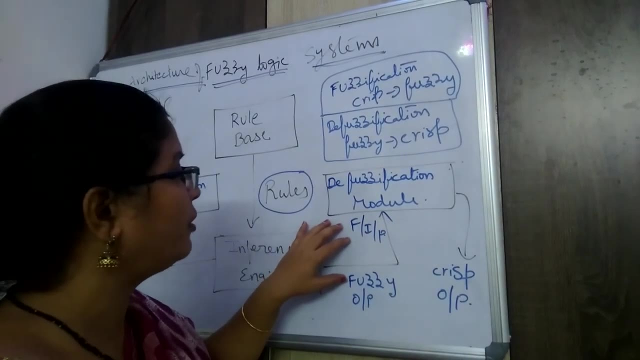 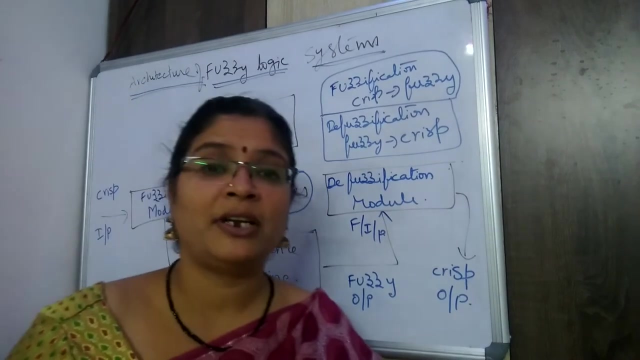 crisp output. So whatever data that we will give as the crisp input using the fudgification module, you can get the fudgy output and whatever data on here you will give for fudgy input, that will be the crisp input. The architecture of the fudgy logic system is designed in a way to transform the data. 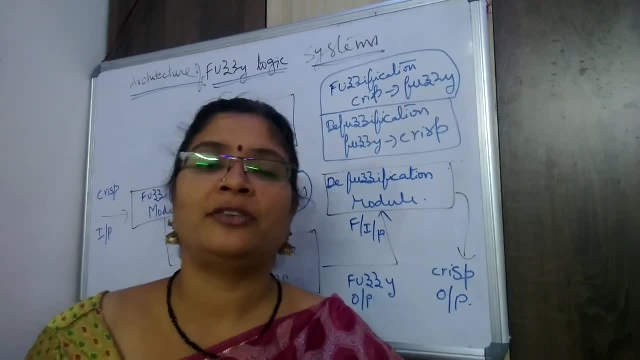 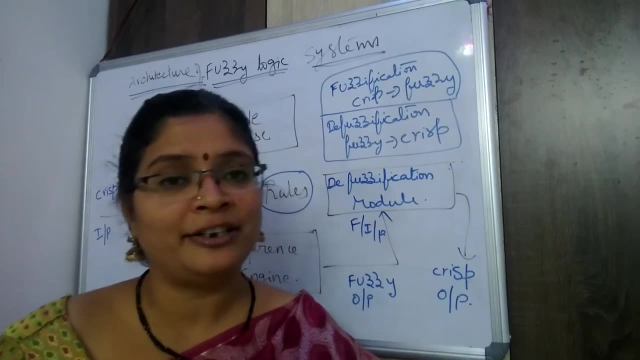 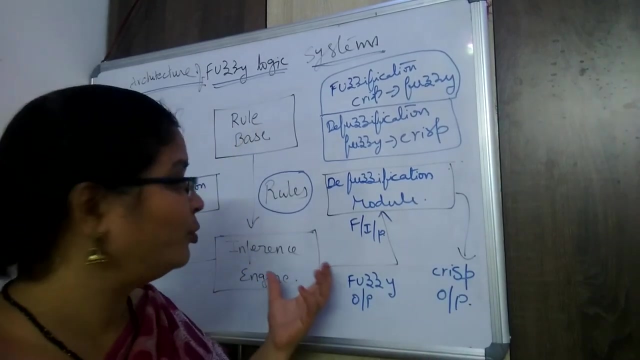 from crisp to fudgy and as well as fudgy to crisp. Not only to storing the data of the rules, not only to storing the set of the rules and conditions based on certain conditions and application of those rules on the respective data, and processing of the rules using the. 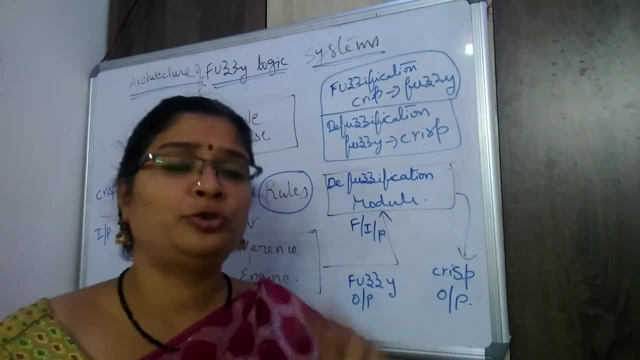 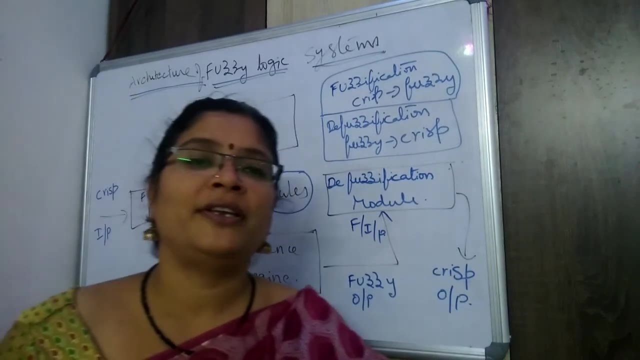 inference engine. it also handles the two important concepts. What are the concepts? Fudgification and as well as the de-fudgification. So these are not the various components of the fudgy logic system. architecture of the fudgy logic system. 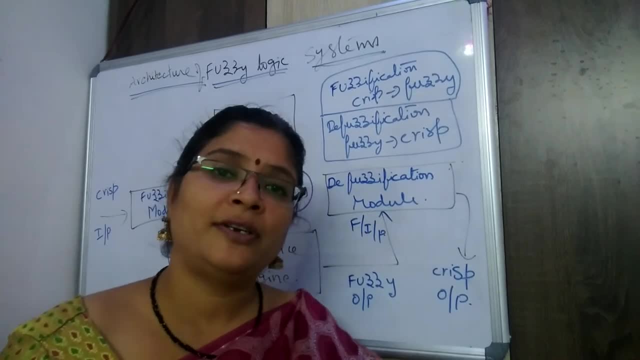 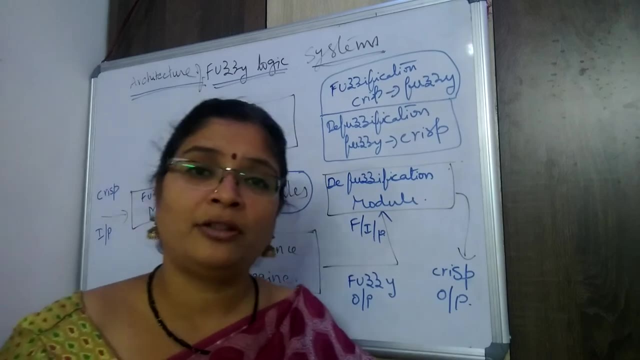 So now we see what are the advantages and what are the disadvantages of these fudgy logic systems, How they are going to be used in the real world scenario and what are the limitations of that. also, now we are going to see So to move, for that I am clearing. 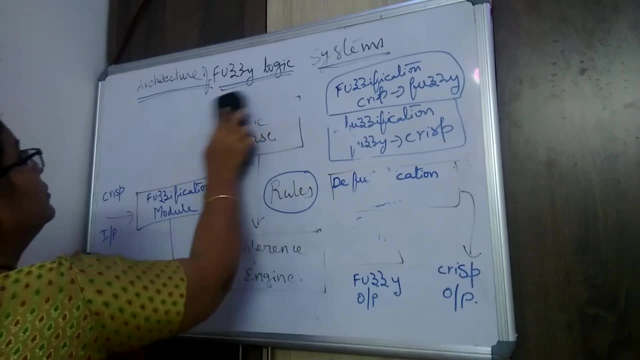 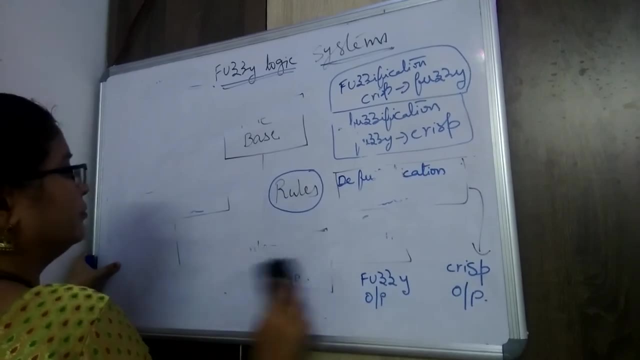 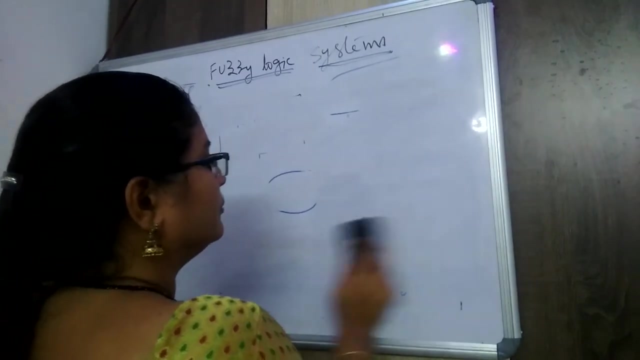 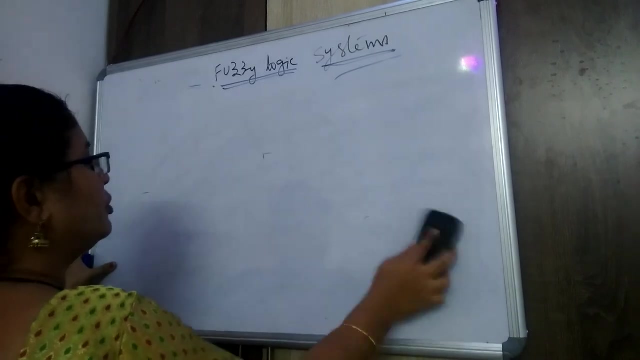 the board. Let us take the advantages first of the fudgy logic systems. Okay, Are the importance of the fudgy logic systems while they are going to be used? Okay, I am talking about the advantages first. So let us take the advantages first of the fudgy logic systems. Okay, Are the? 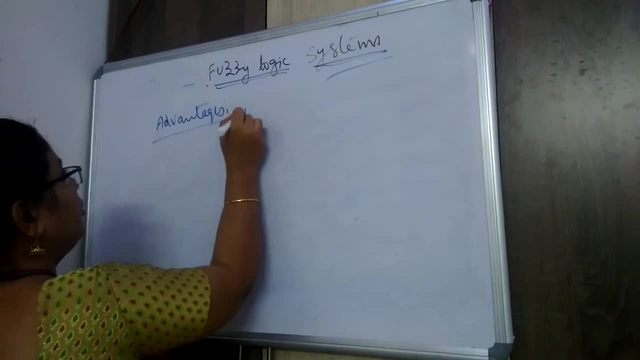 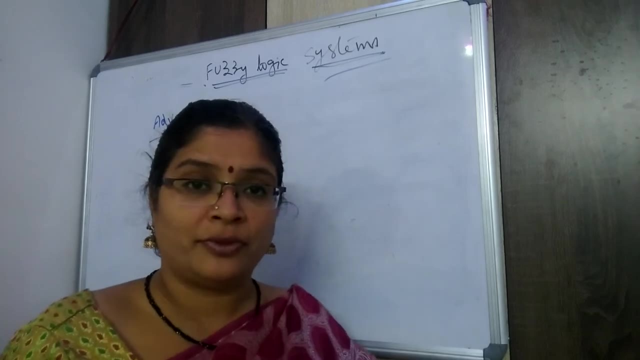 biggest advantage of the fudgy logic systems? Okay, Are the biggest advantages of the fudgy logic systems? Okay, Are the best advantages? So what are the best advantages of the fudgy logic systems? okay, So the first best advantage of this fudgy logic systems is these are used to design decision support systems and these 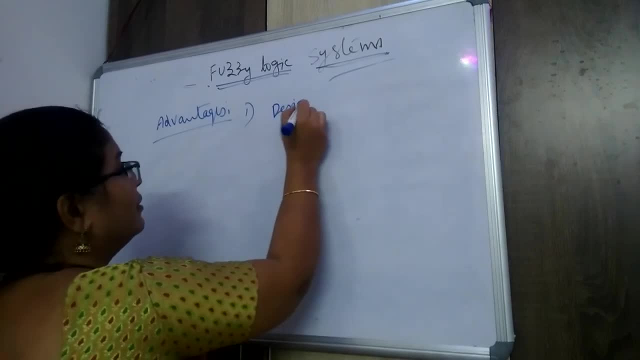 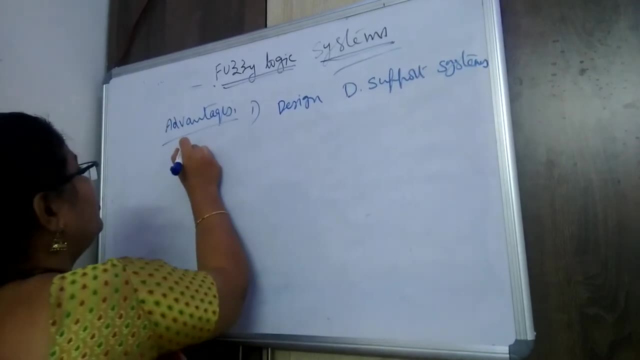 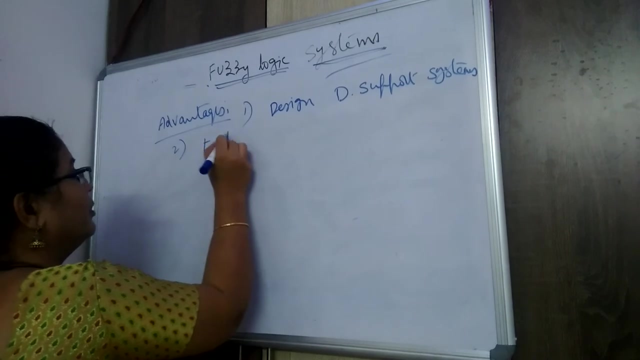 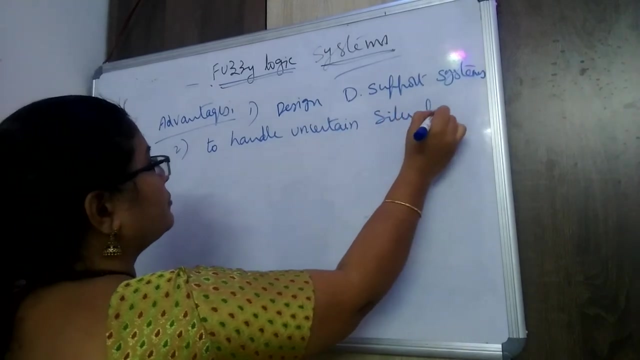 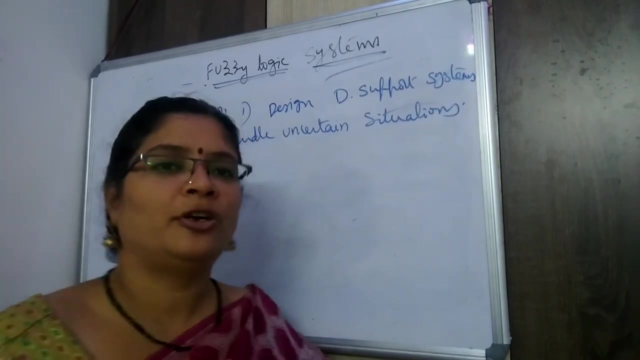 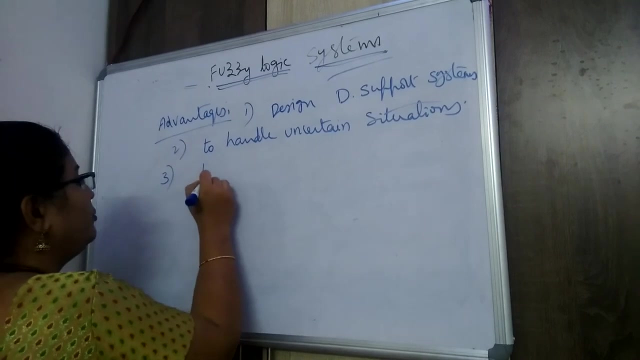 are used to heal in These advantages. we all of you know what that is. to handle the unsettling And uncertainty can be successfully handled with the help of the fudgelogic systems, okay, And to design very good and efficient fudgelogic systems. 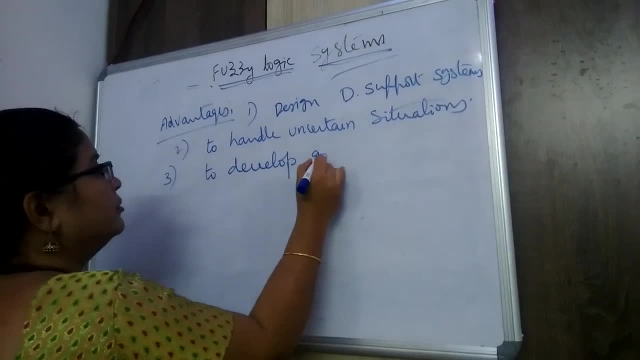 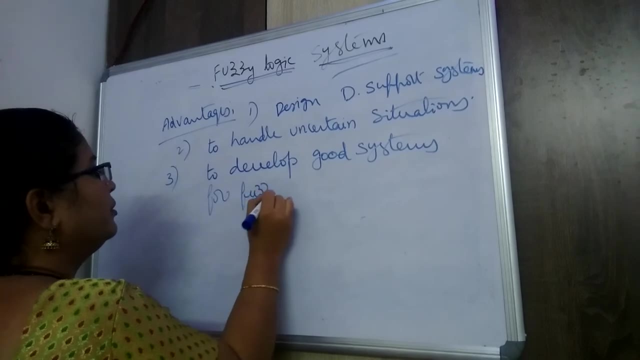 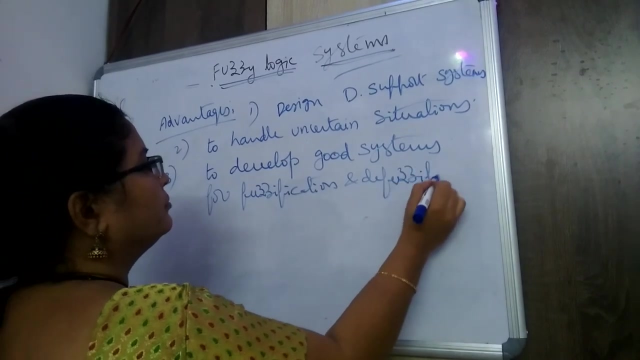 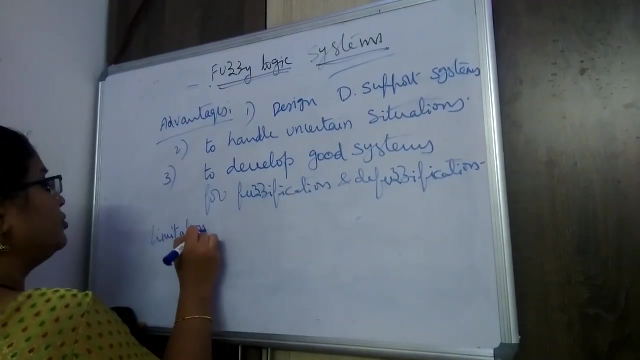 And to develop good systems for fudgification and de-fudgification like that. we are having so many number of advantages of this, but what are the limitations? coming to the limitations of fudgelogic, As we know, for each and everything there will be some limitations. 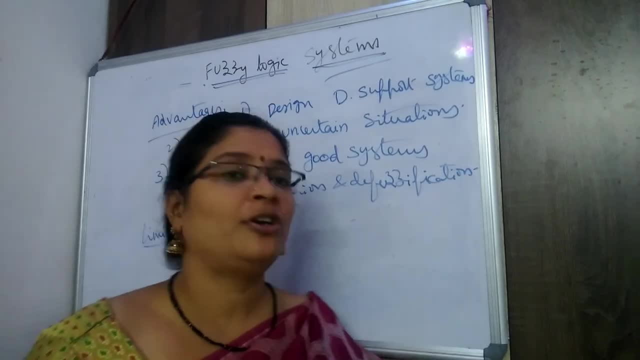 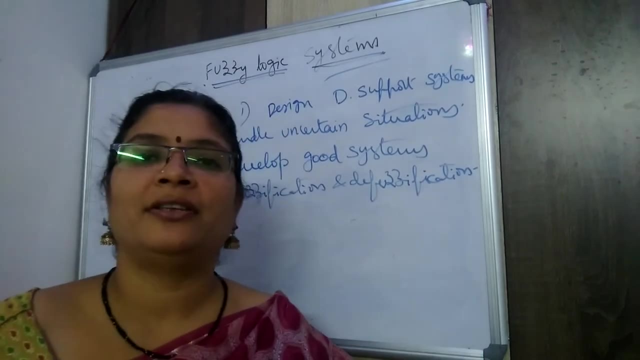 Okay, So all the limitations will be there, obviously. So the fudgelogic is also having its own limitations. So what are the limitations Now we are going to see here? the first limitation is: it's not at all accurate. 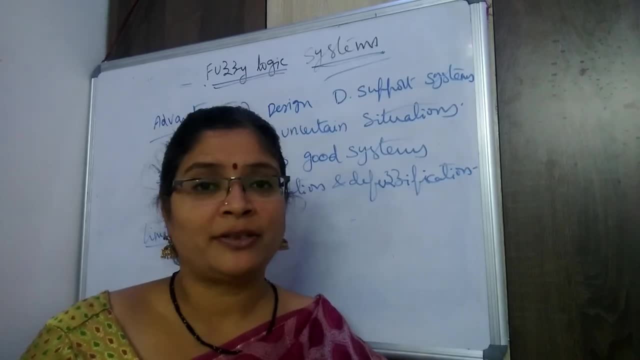 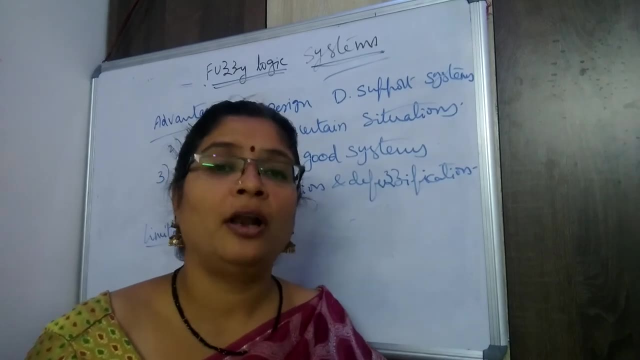 Okay. So whenever we are developing such a kind of the systems which require accuracy, high accurate systems, this fudgelogic is not at all helpful. Okay, So, not accurate. This is the one biggest disadvantage of fudgelogic systems. 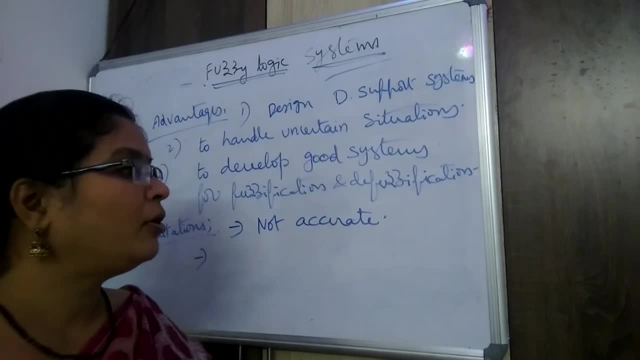 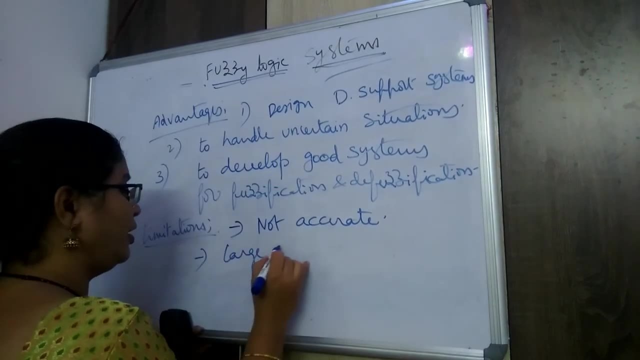 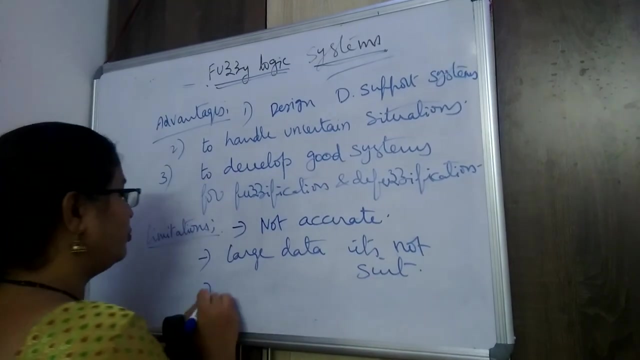 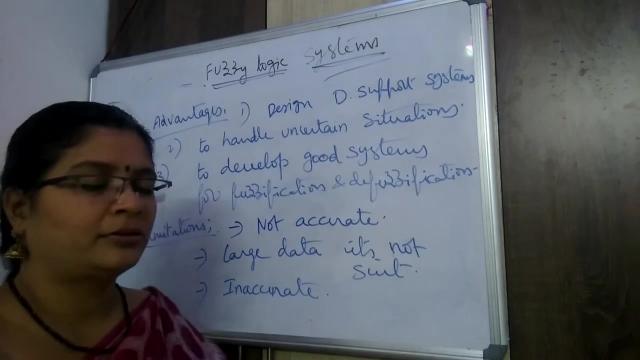 Okay, disadvantage of this Whenever you are going to handle the large data. more amount of the data is also not useful. okay, For large data, it's not suit. okay, So we can say it's somewhat inaccurate comparing to other methods which handle the uncertainty like artificial. 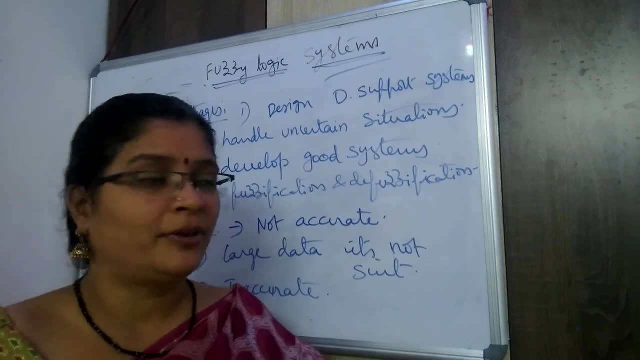 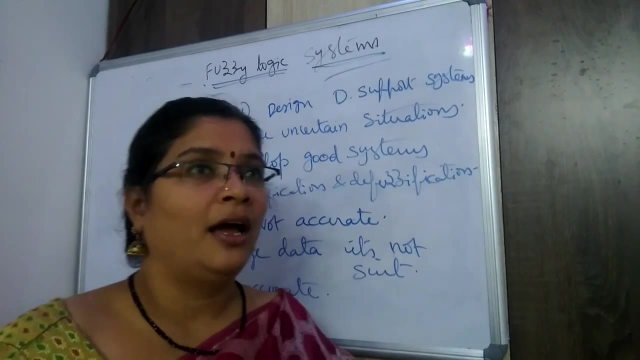 neural networks and other kind of the things, whatever are there For such a kind of the systems for comparing to these fudgy logic systems, for such a kind of the systems like artificial neural networks and so many number of the things. this is somewhat disadvantageous.